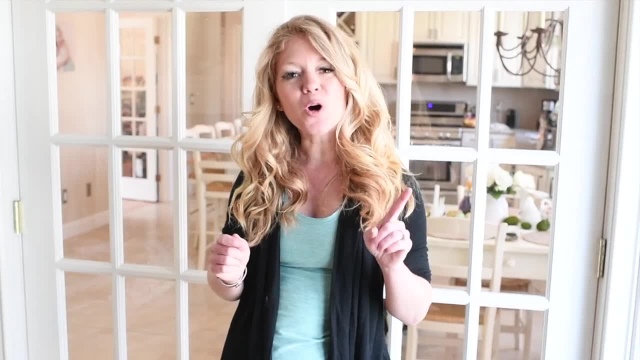 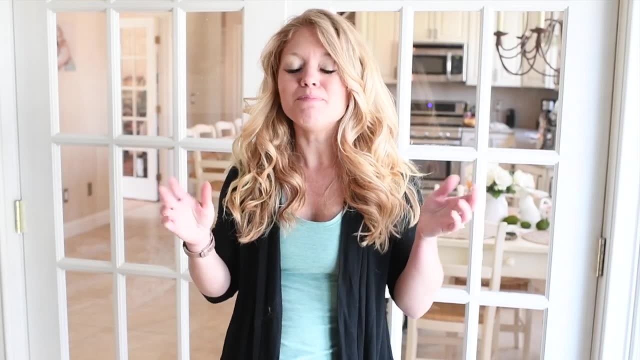 Okay, so light is the number one factor in photography. The cool thing about photography is it allows us to pay attention in a way that maybe we wouldn't have looked at things before. In this lesson, you're going to learn how to look for the light in different natural light. 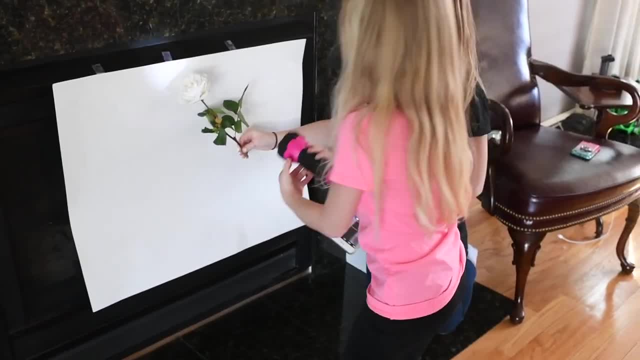 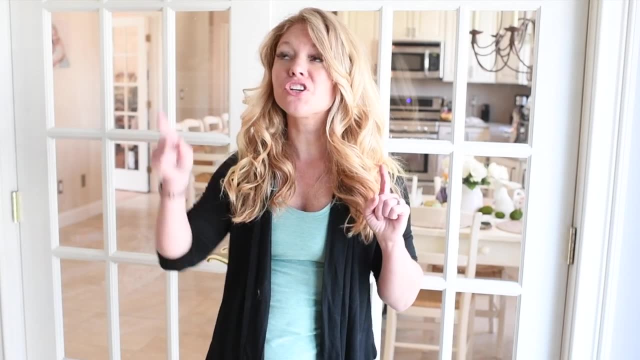 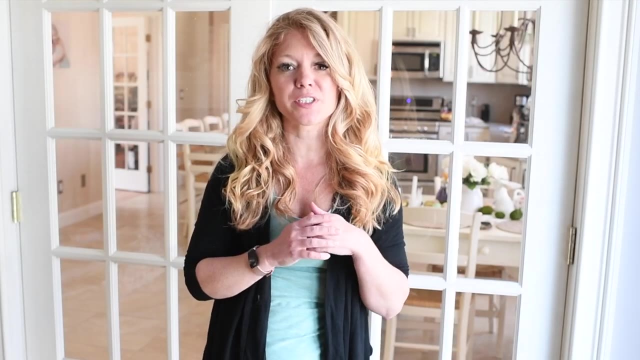 scenarios and we'll actually play around with using some artificial light like flashlights or lamps or whatever you have on hand. It's important in a lot of these exercises to make sure that the overhead lights in your house are on So that you can really see the lighting patterns coming from natural light sources like windows. 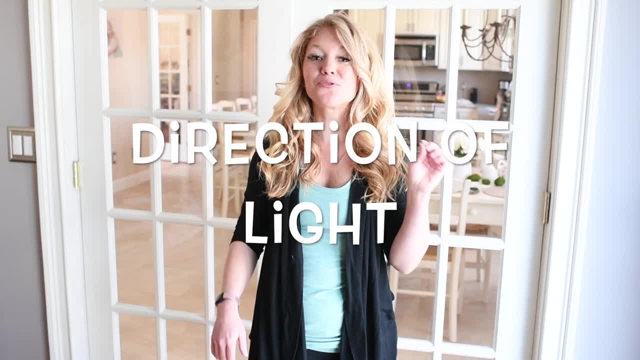 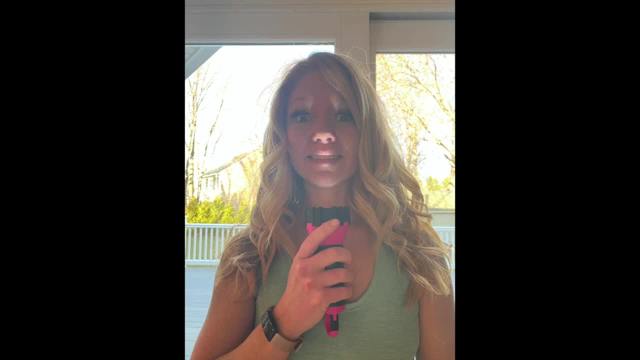 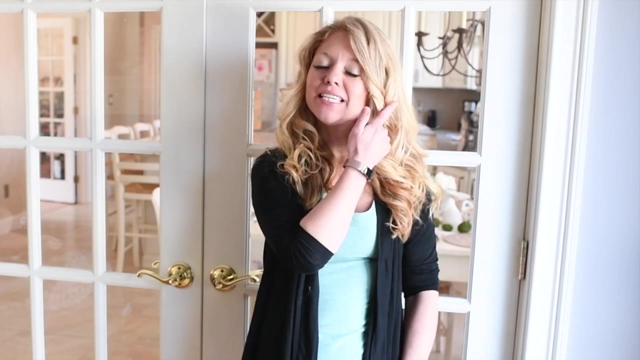 and doors and things like that. So the first thing we're going to talk about is the direction of light. So that's, where is the light coming from? See, this type of lighting looks really different than this type of light. So when you look at an object or a person, you can see where. 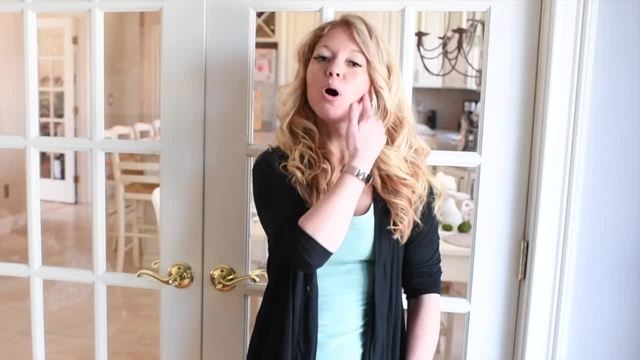 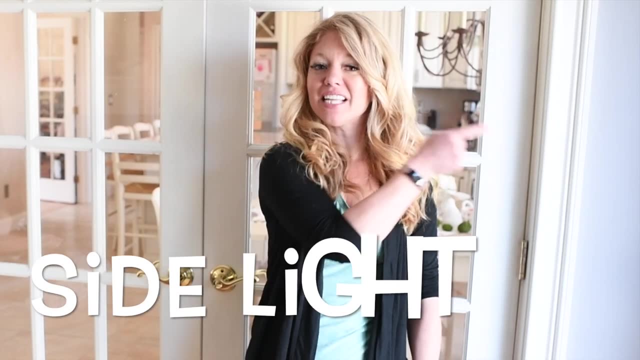 the light is coming from, the direction of the light, by what part of the object or the face is light. So you can see where the light is coming from, the direction of the light, by what part of the object is lit up. So right now I'm standing in side lighting because the light is coming from. 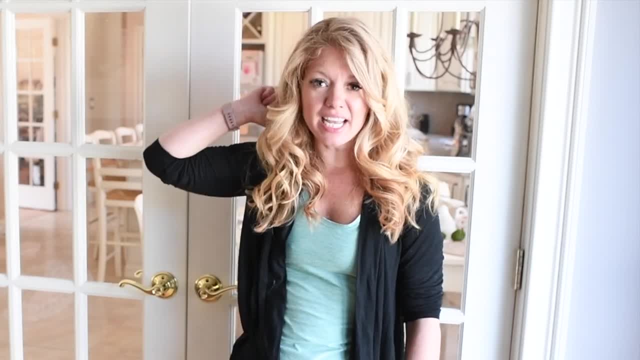 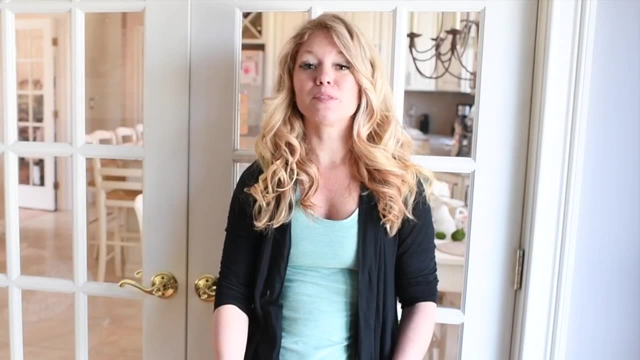 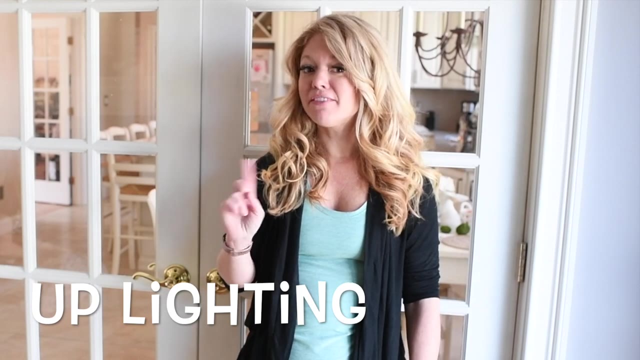 the side. If you have overhead lights or you're standing outside on a sunny day, that would be top lighting or down lighting. If you have a light source beneath you, like my flashlight, this is called up lighting or lighting from beneath. There's another element of light that 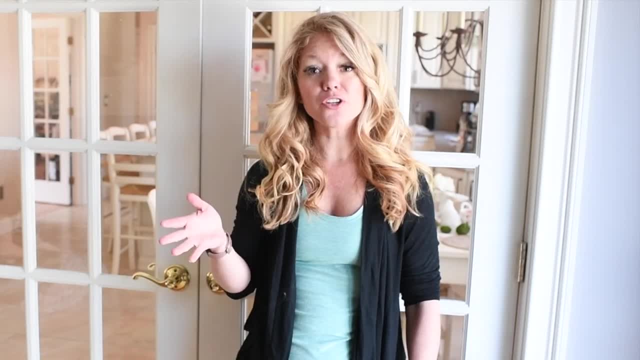 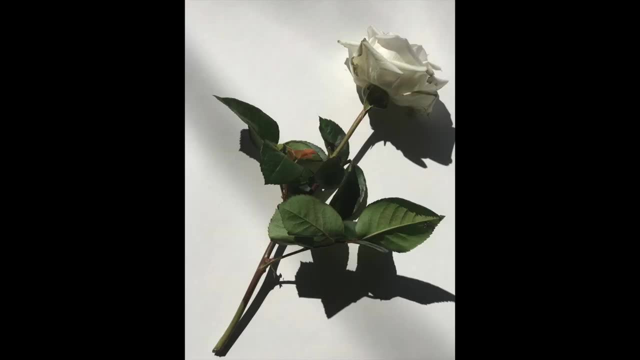 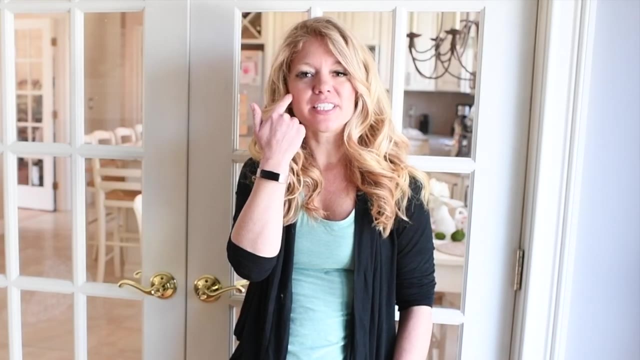 you want to pay attention to, and that is whether it's hard or soft. So hard lighting is when it's really dramatic change, So it would be like really bright on this side and really shadowy on this side. Soft lighting is when it's a really gradual transition between light and dark. So we 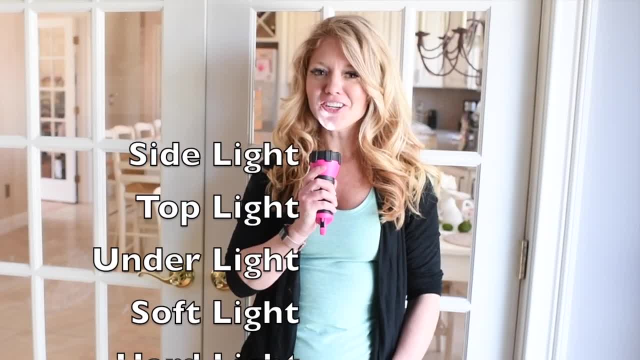 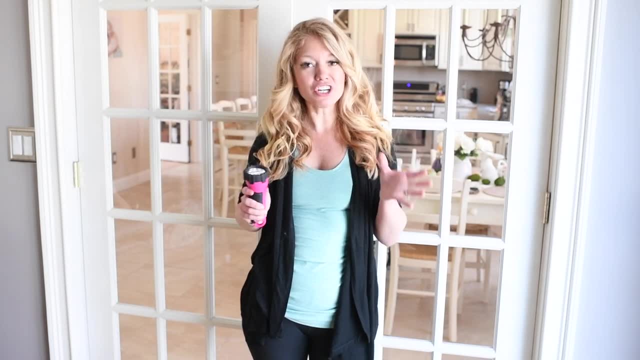 talked about side lighting, top lighting, under lighting, and we talked about soft and hard lighting. So now we're going to try out what these types of lighting looks like on different objects or people, depending on what you have on hand, to really learn these concepts and practice these. 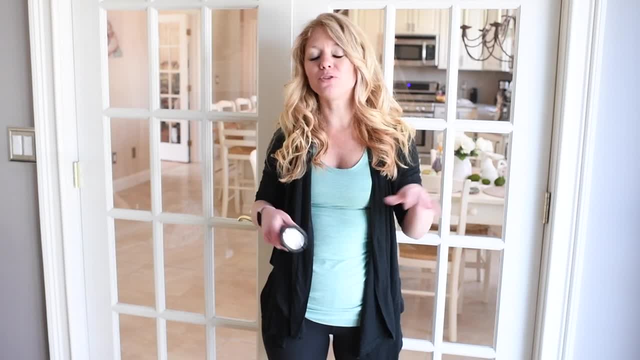 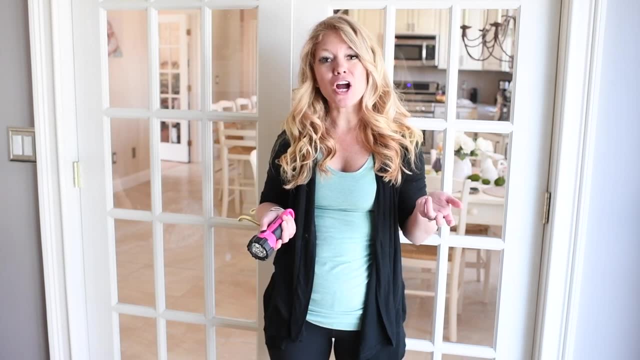 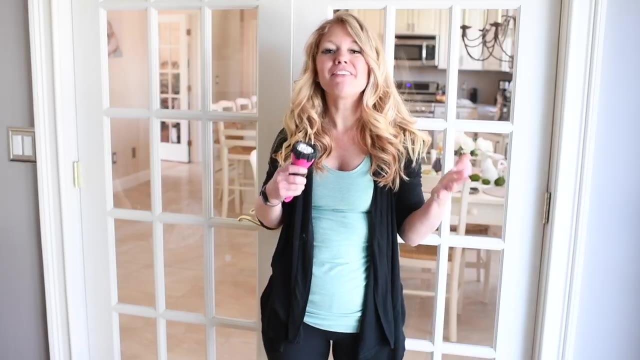 concepts. With photography, it's not just about trying to create the next masterpiece. It's really about the process, enjoying the process. The way to get better at photography is by experimenting and doing. You learn as you go. So have fun with these, be silly, be playful and creative. 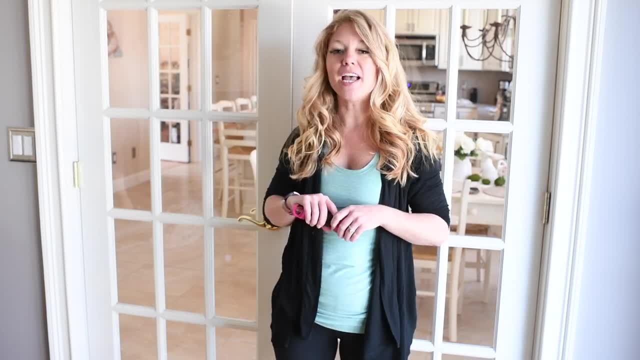 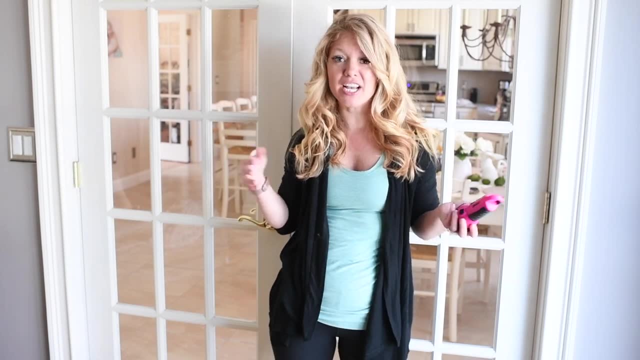 and see what develops. Okay, so in the activity we are going to choose either a favorite object, or it could also be a person, a subject, a model, Somebody, a sibling or your parents or whatever, And we're going to bring them into all different. 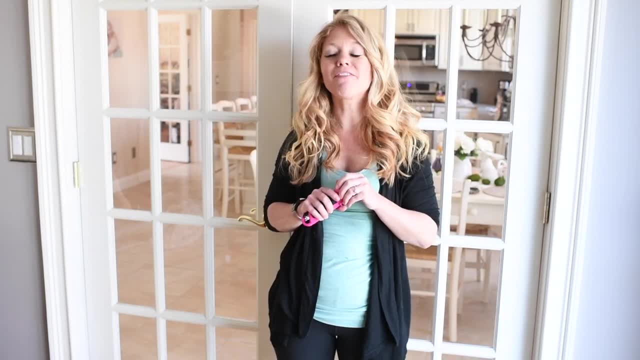 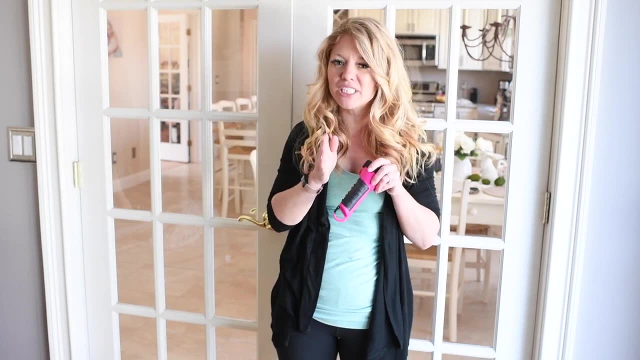 spots of light throughout the house and take a photo of it. We want to find as many different light sources as possible in your house And, of course, we want the overhead lights off for these so that you can really see the patterns of light. Okay, so you guys can each find your object. that 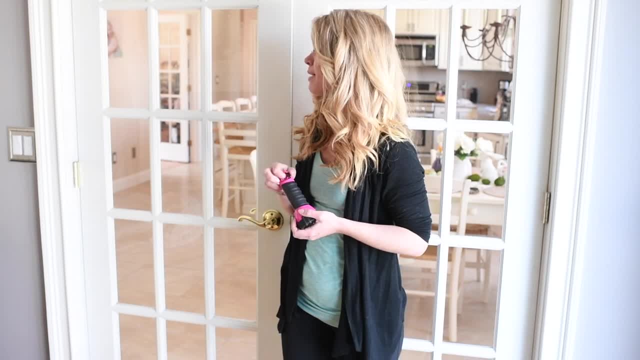 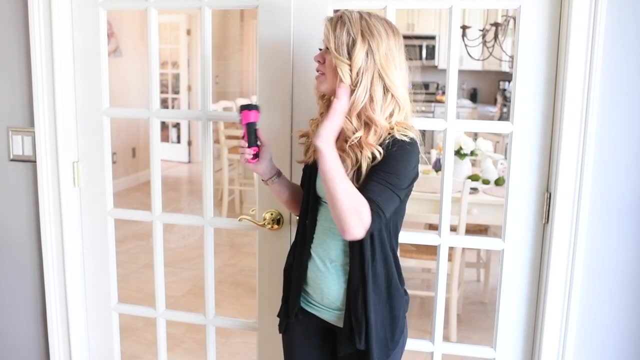 you're going to photograph. So you pick anything you want. Grant, go pick your favorite toy Girls. you can pick a toy. You can pick something decorative You can pick. you can photograph each other if you want to, Alright, so my kids are going to do this. 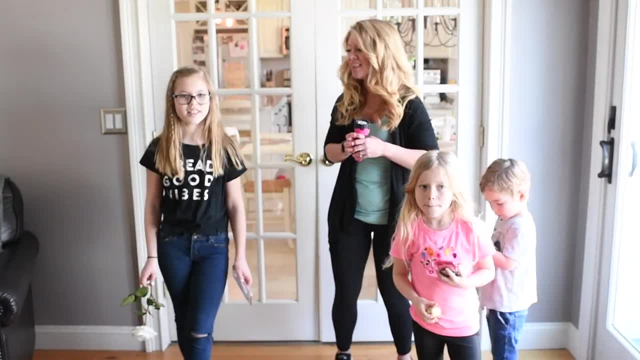 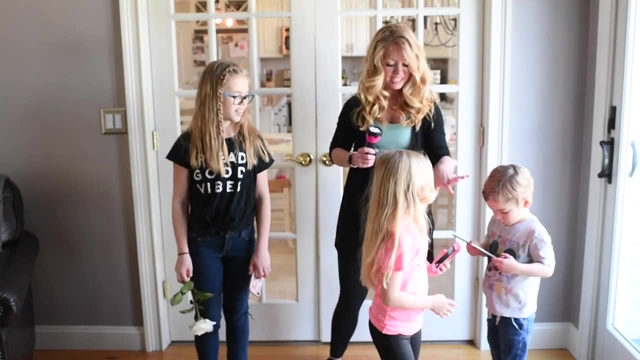 activity too. They all have their objects. So come on in guys. They are ages 11,, 7,, almost 8, and 4 and a half, So they have their. Grant has an iPad and Grace has an iPod and Juliana has. 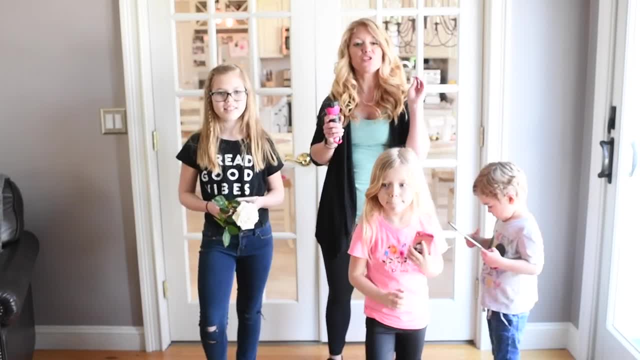 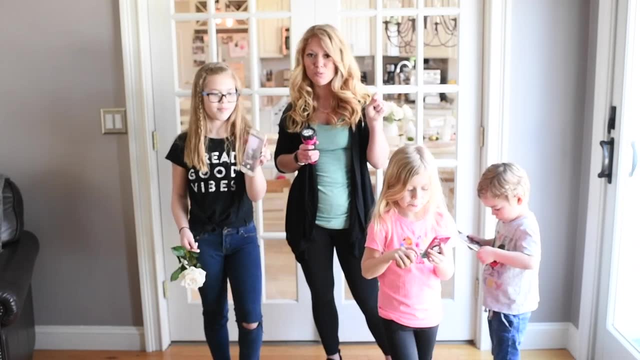 an iPhone, So any device will work for this. So you want to go into the camera- any device with a camera, So you want to go into the camera. If you have portrait mode, try doing this on portrait mode. Portrait mode on the iPhone is going to blur the background for you and create 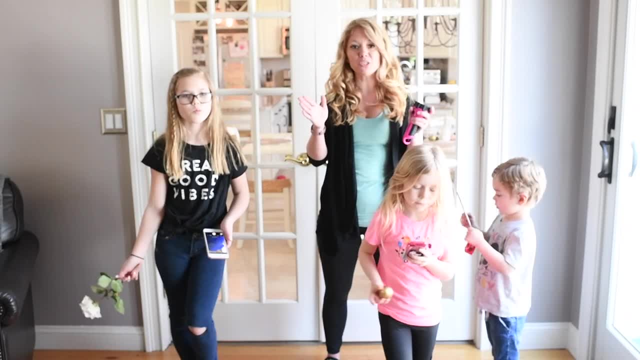 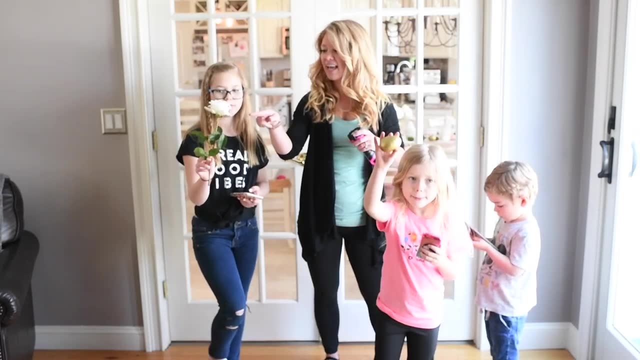 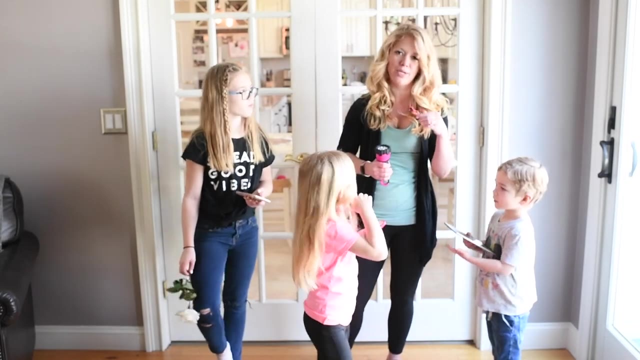 a more professional looking photo. If you want to photograph a person, you can just photograph a sibling or something, or you can go get an object. So they've all got objects. So Juliana has a rose and Grace has an egg from Easter decorations and Grant has a toy car. Lightning McQueen. 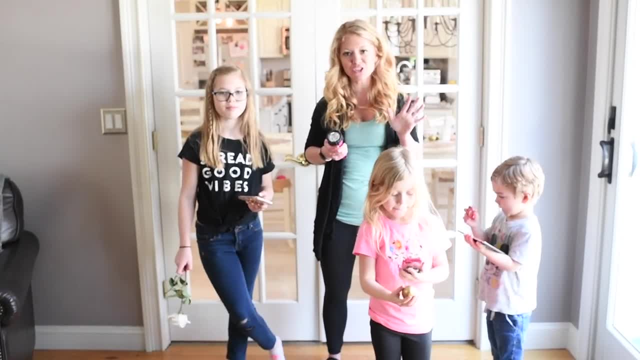 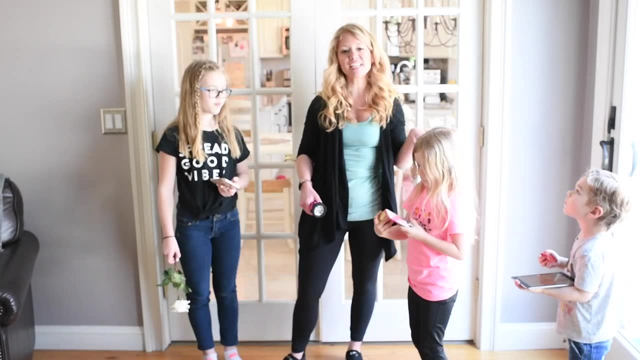 We're going to now practice with the different types of light, taking pictures in the different types of light using these objects. If you want to, you can create a little backdrop for yourself, like a white piece of paper or a white piece of poster board that you can put down in each room. 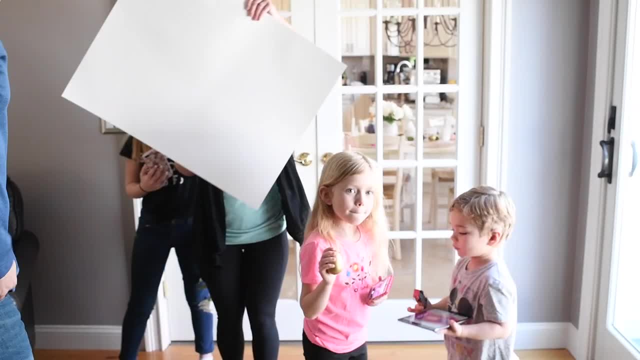 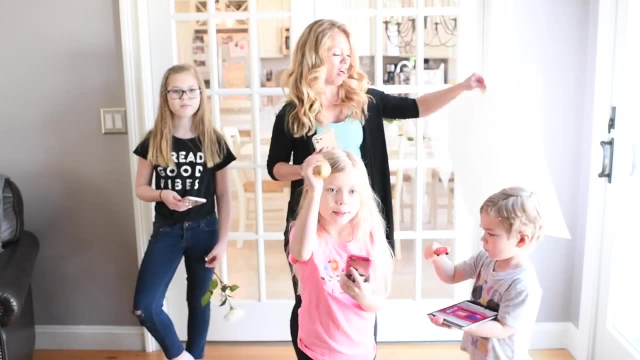 so that you can really see what the light looks like. Okay, Susanna's got a poster board for us. So if you have a solid background like some computer paper or poster board, you can do it on that, or you can just photograph on any. any floor is fine. 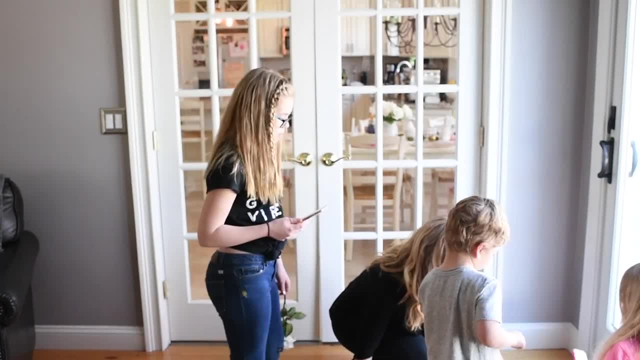 Okay, So we're going to put this down here and let's start with Grace. Okay, So I'm going to take a video from the background. So I'm going to take a video from the background, from above, so you guys can see this too. So Grace is going to lay down her egg and move it a little. 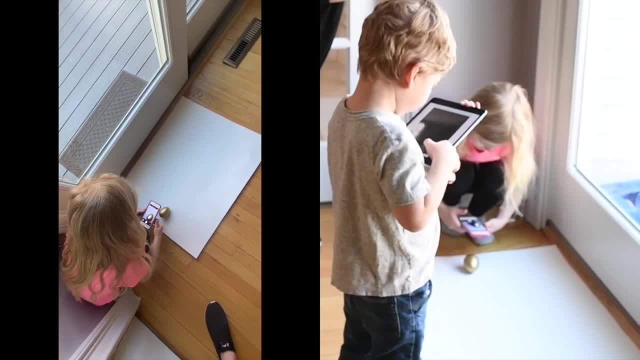 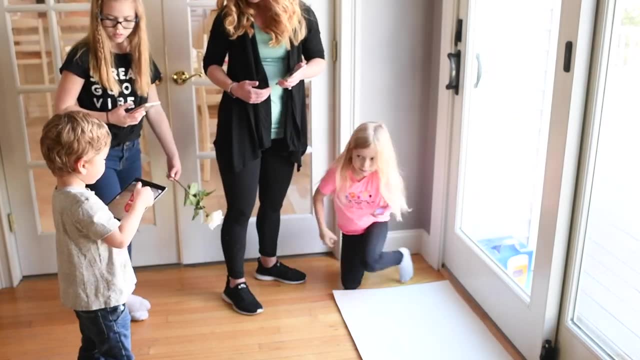 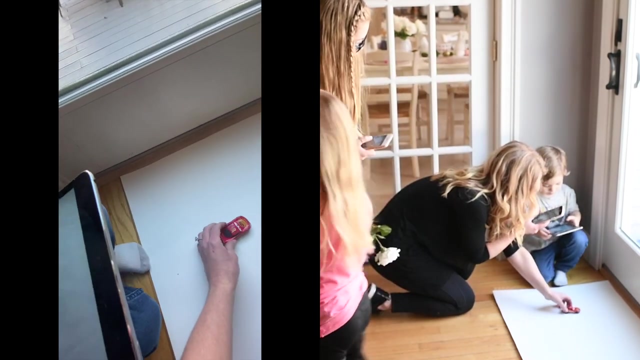 bit more towards the front. Yeah, there you go, And then she's going to center the egg. That's a really good example of side lighting. Okay, Grant, you want to do your car? Okay, And then come down close. You want to zoom in on him like this? Okay, So let's turn him so that he's 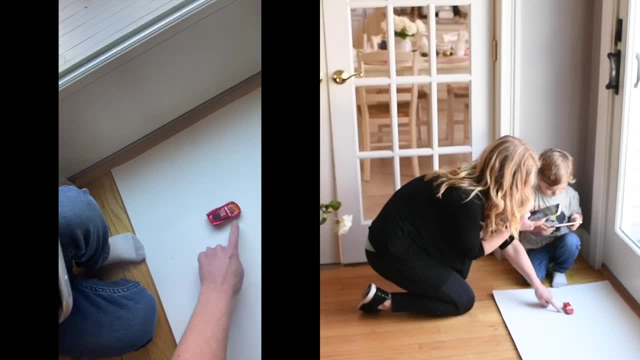 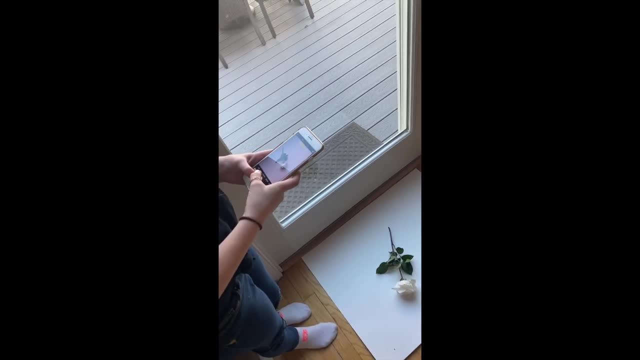 so the light is coming on the side like this. You see where the shadow is on the side. So she's in portrait mode, so she has to stand up a little bit further. You can try it outside of portrait mode too. Let's try opening the door. 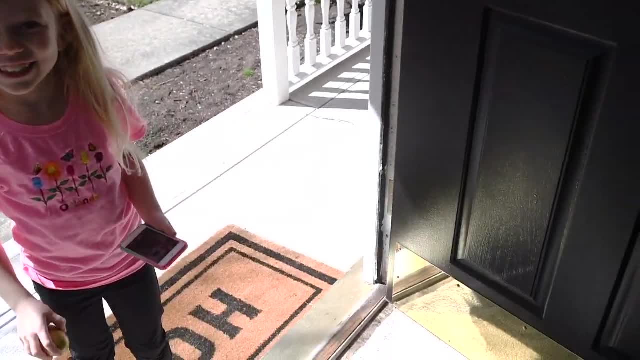 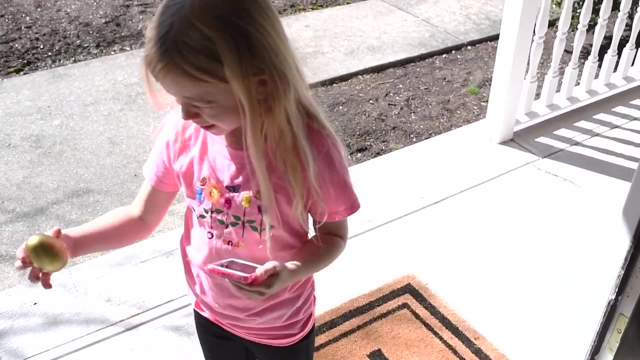 Do you want to get the poster board and put the poster board down? Yeah, It's very bright today, Very bright. So is that hard light or soft light? Um, I think it's hard light. It's closer to the sun, so it's- um, It's hard light, yeah, Brighter. 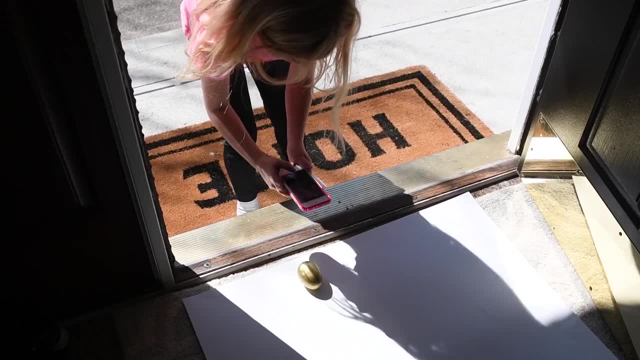 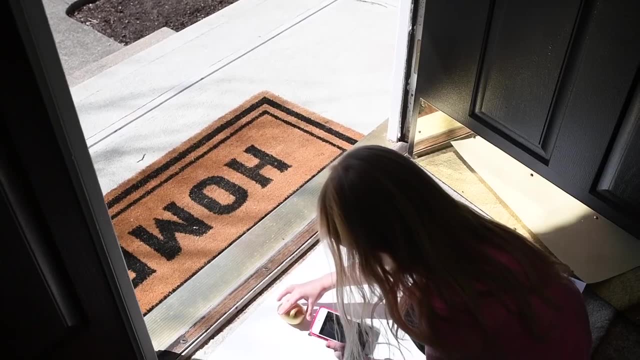 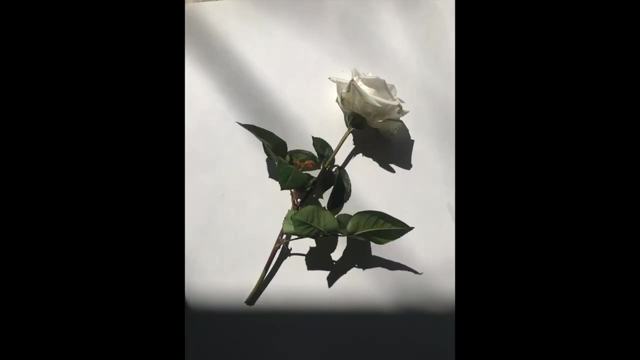 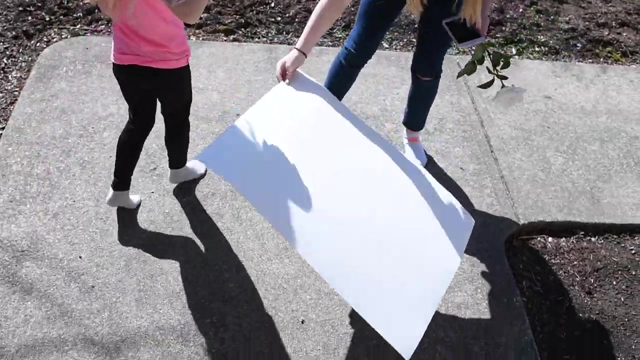 So, Grace, because your shadow is right there, maybe try taking a picture of it from the other side. There you go. So what type of light? do you think that was A hard light? Yeah, definitely. So what direction is this light? This light is coming from almost pretty much straight ahead. 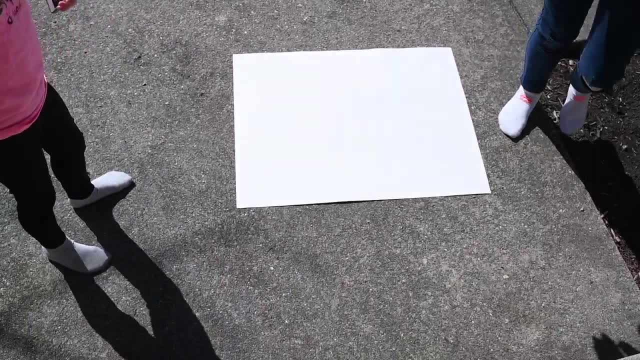 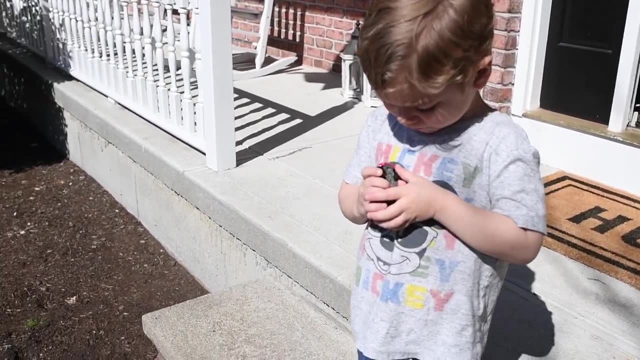 so I think it's on that side. Yeah, almost top light, a little to the side. You can tell by the shadows. Grant, do you want to take a picture of your car out here? No, Okay, The egg's tough. 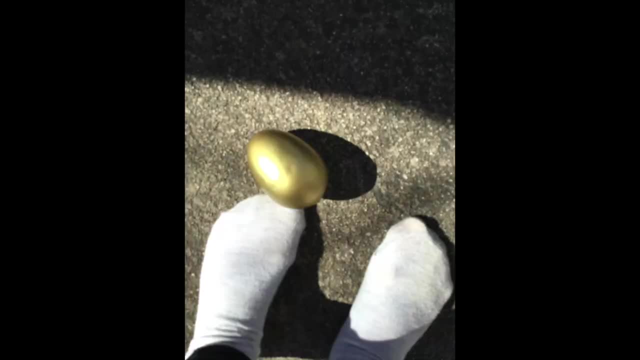 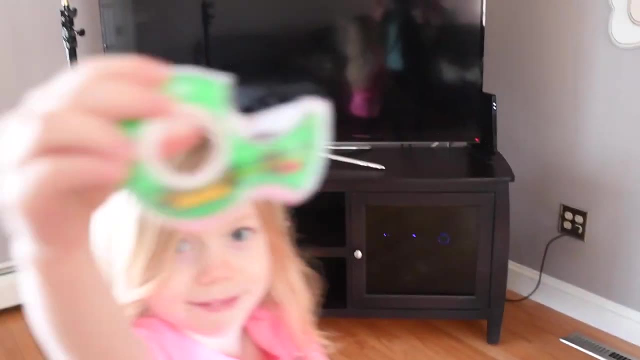 because it rolls, but then your feet are going to be in it. It won't work. Oh, thank you. Okay, so we're going to try to. why don't we tape this? We're going to tape the poster board to the fireplace. Okay, so we're going to try to. why don't we tape this? We're going to tape the poster board to the fireplace. 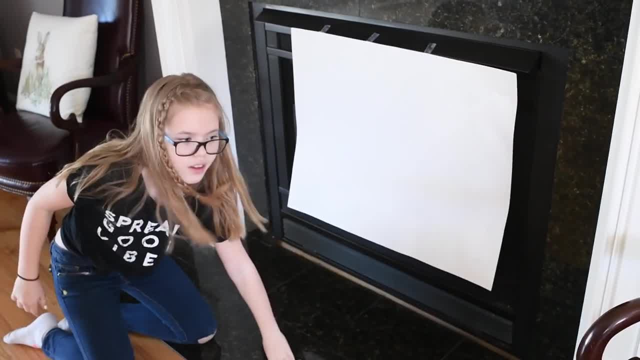 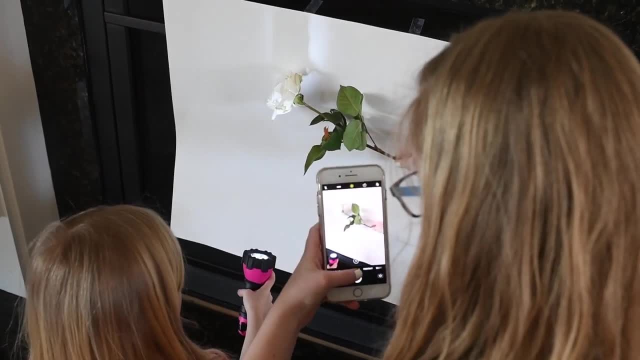 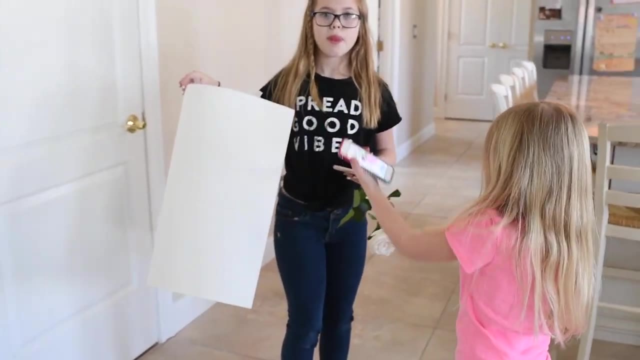 All right, so we're creating a little background so we can try out under lighting. The lights are too bright in here that you can't tell. Should we go somewhere darker? Yeah, Okay. Hmm, where can we find a dark wall? Oh, in the basement. Oh yeah, We're literally right in the 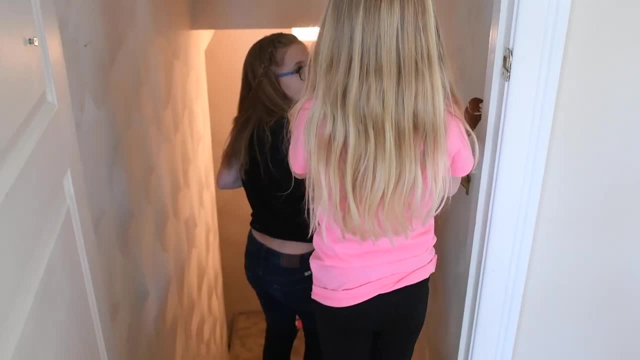 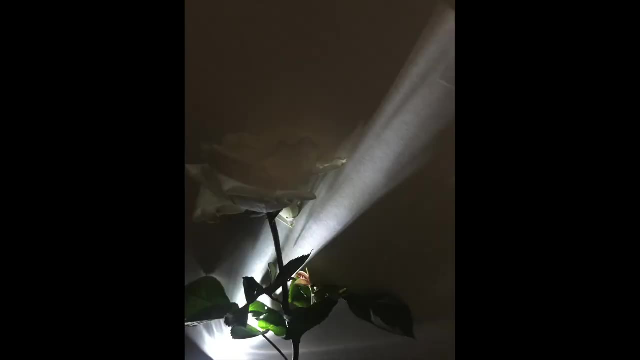 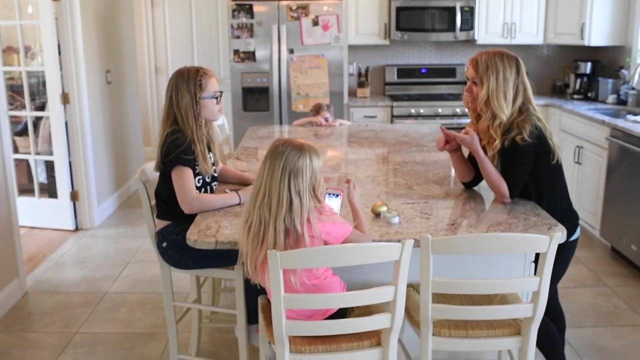 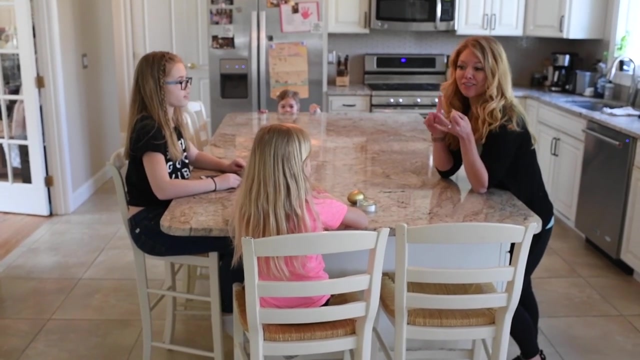 bottom Down low. Yeah, keep that light off, though. Let's just do the bottom of the stairs. Yeah, Okay, so we got top lighting, We got underlighting. We got side lighting. We got hard light outside, We got soft light inside. right Now, what I want you guys to do is go. 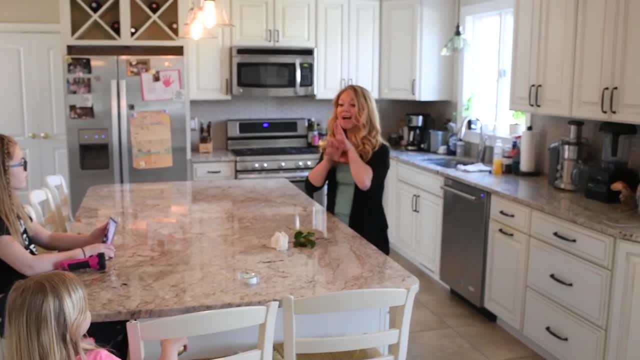 around wherever you want and place your object down and try to just get creative pictures. so you already have. You know how the light works. You know the different directions of light. Now just walk around the place and try to just put your light in there, And then you can go around the corner. 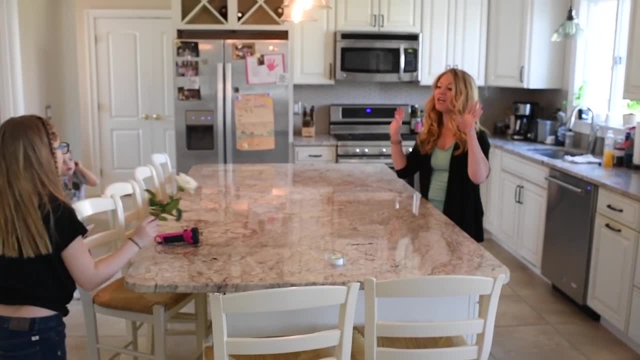 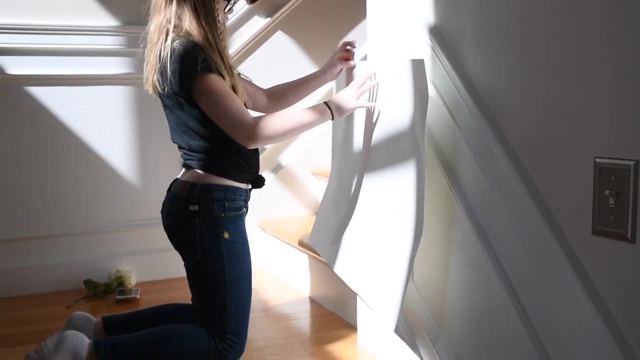 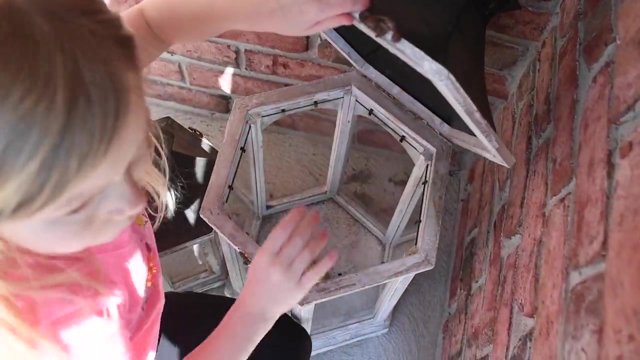 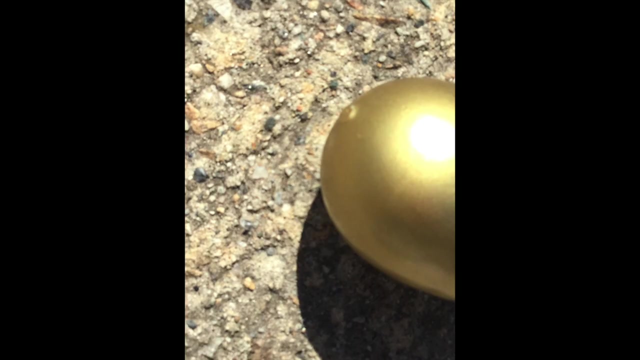 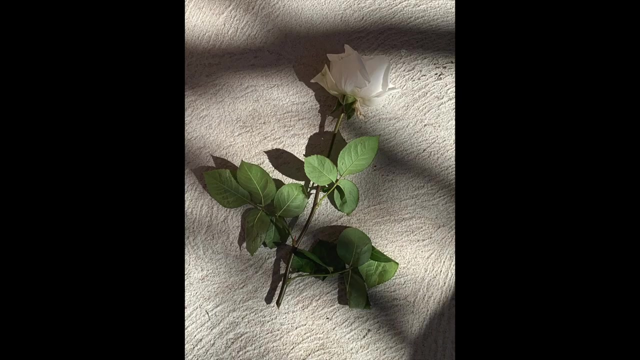 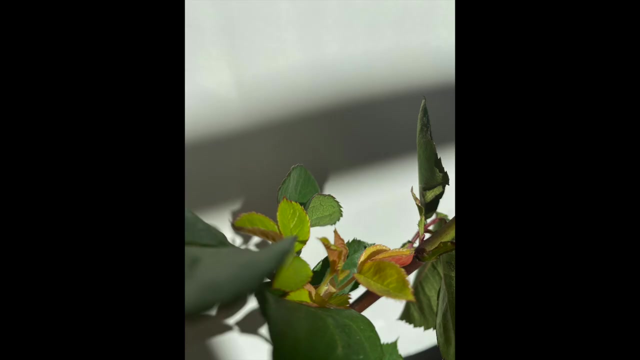 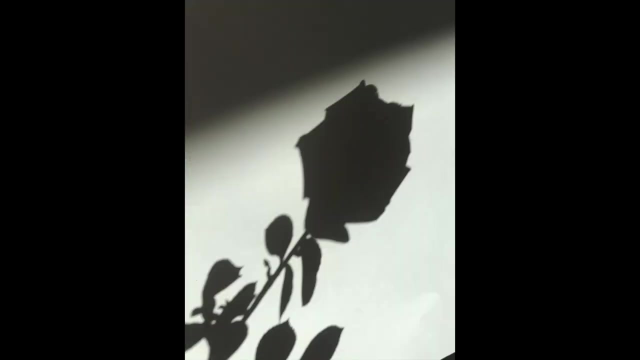 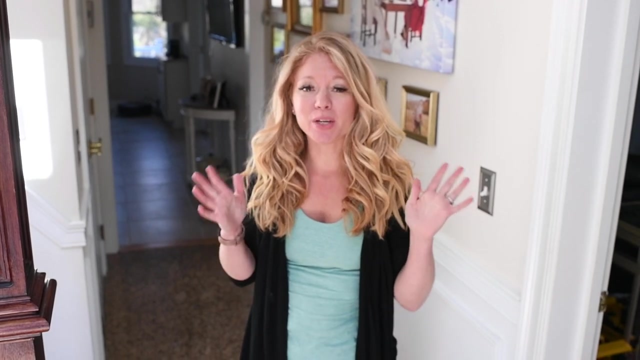 You know the different directions of light. Now just walk around the corner and try and get a better picture. Okay, house or even outside- and you can take pictures of your object in all different types of lighting. all right, so we got a lot of really cool, creative pictures. we learned the directional light and 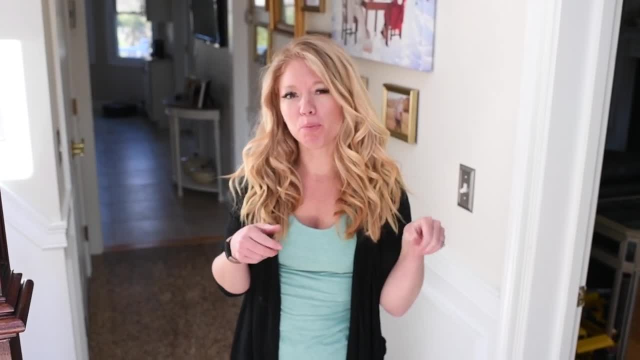 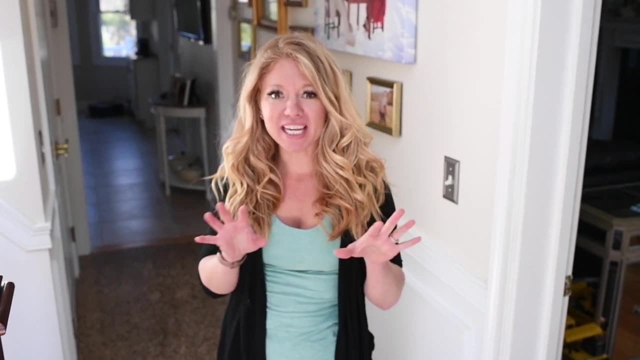 hard and soft light. i found the kids were probably a little bit more bored with those pictures. and then when i said now you go have fun and i'm going to show you how to do that and be creative and find you, find your own light and shadow, i'm like super impressed with the. 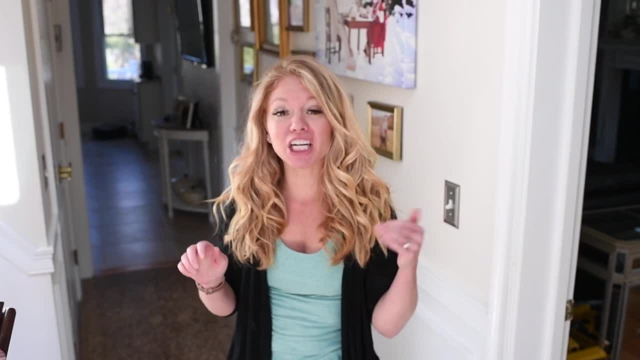 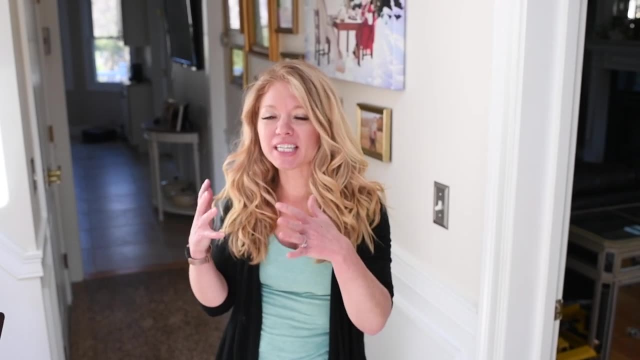 pictures that they got when they got to just go and explore. so really encourage kids. or, if you're older kids you're watching, be creative. stick that either the object or the portrait, if it's a person. try to put them into unusual places. look for patterns of light and shadow that you can kind. 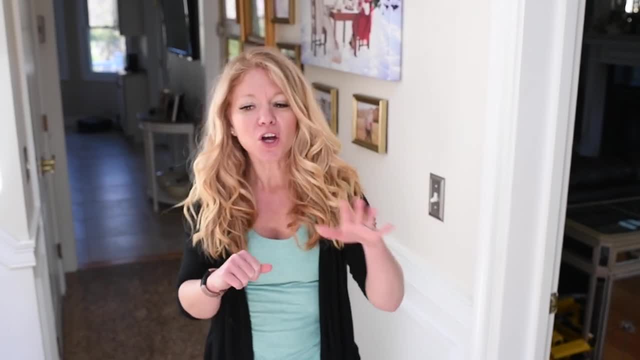 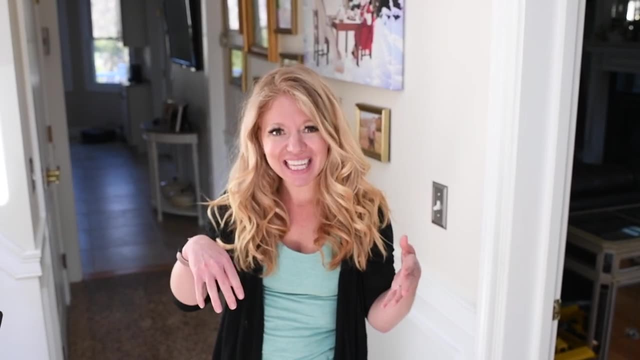 of play around with whether you're finding light and shadow on a wall or, if you're out, if you're able to go outside and get some outdoor pics. one of my favorite ones was the one that grace did inside the lantern. i thought that was such a cool, creative.